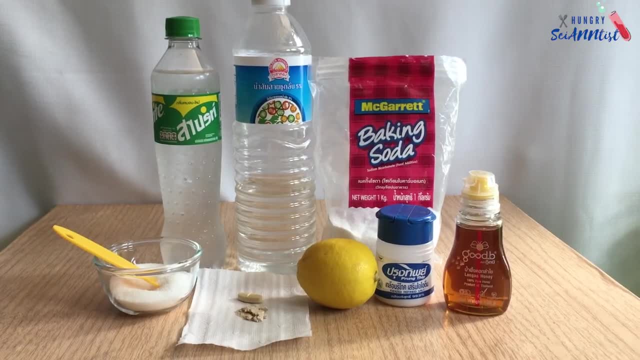 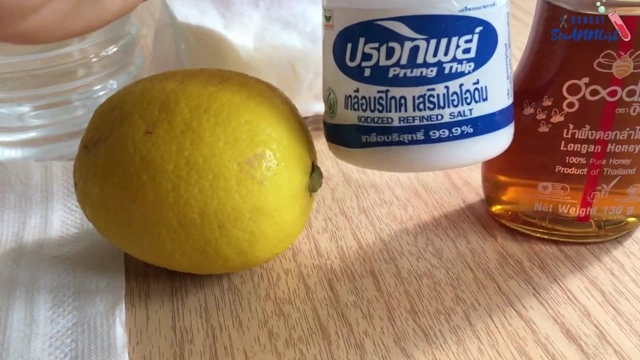 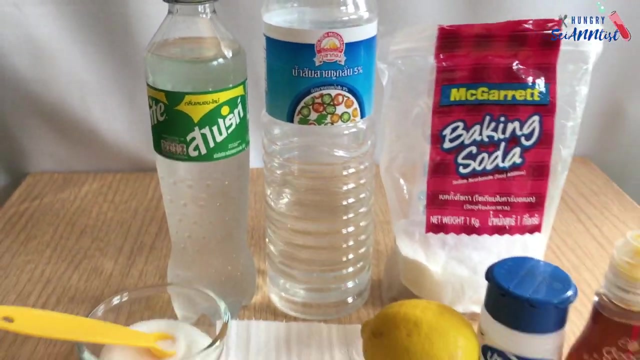 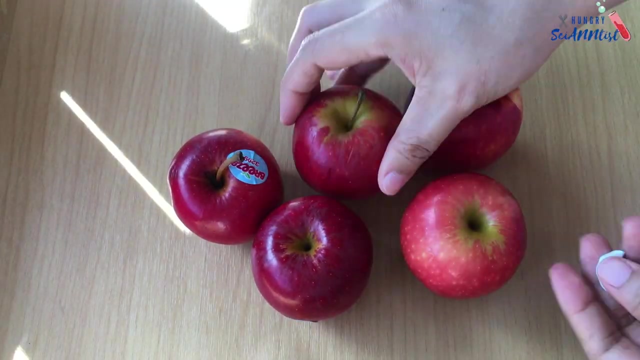 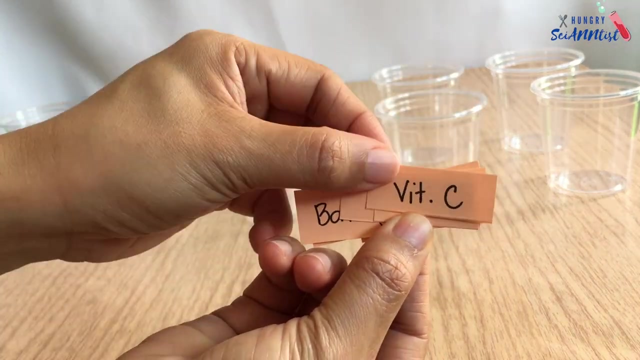 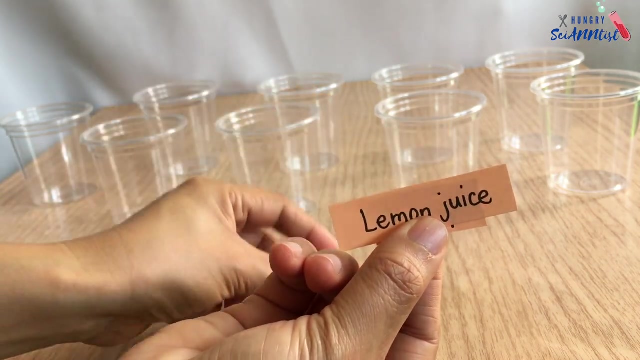 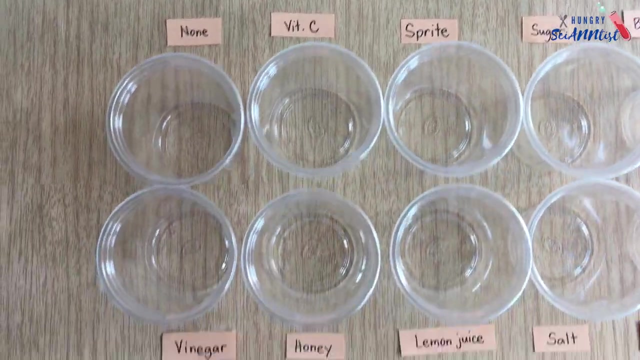 What is the best way to keep apples from turning brown? In this experiment I tried different solutions to keep the apples from turning brown. First we must prepare our cups and the labels Pour 1 1⁄2 cup of water. 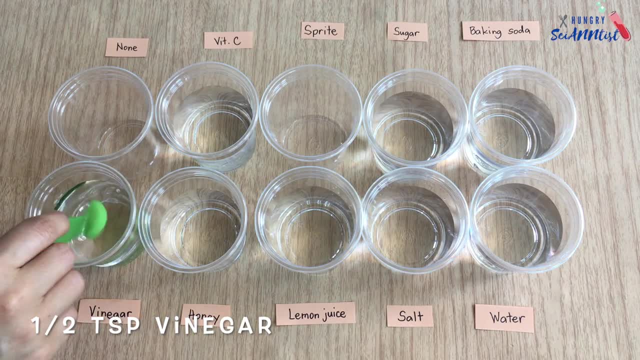 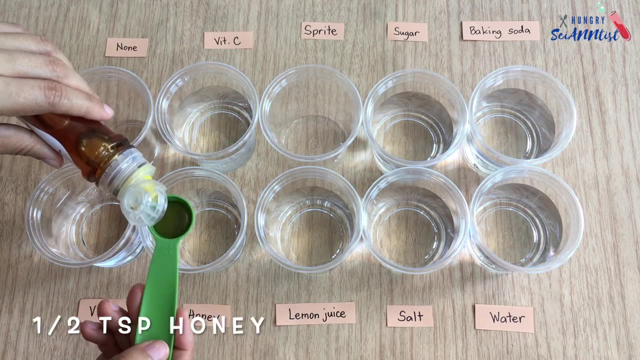 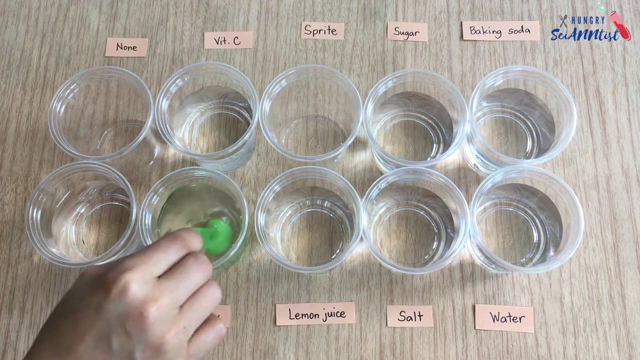 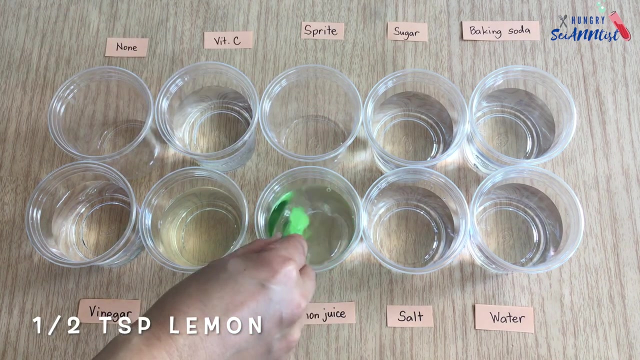 To make the solutions. first, we will add 1⁄2 teaspoon of vinegar. Add 1 1⁄2 teaspoon of honey. Add 1⁄2 teaspoon of lemon juice. Add 1⁄2 teaspoon of salt. 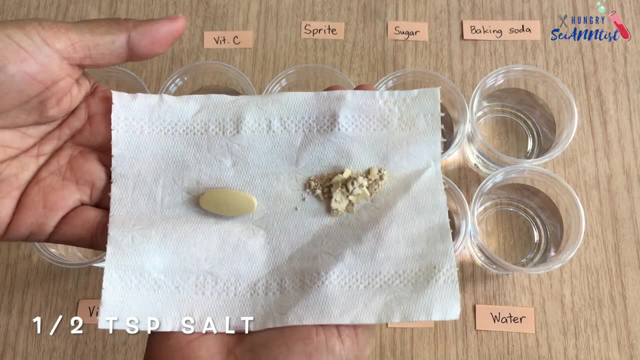 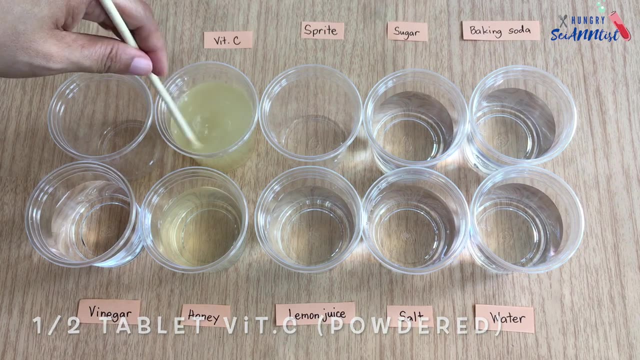 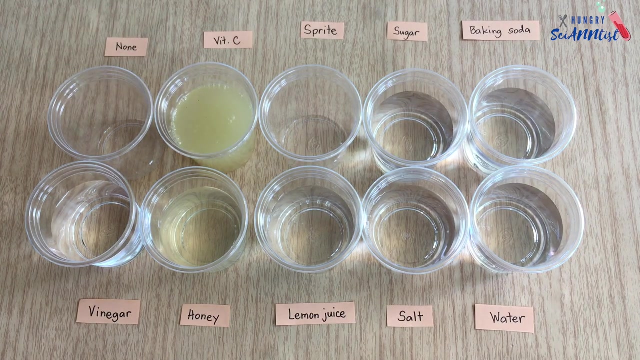 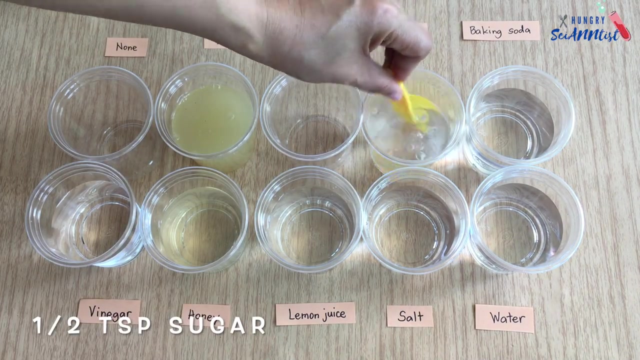 Next is just plain water. Add 1.5 teaspoon of sugar. Add 1.5 teaspoon of lemon juice. Next, half a tablet of vitamin C. Add 1 1⁄2 teaspoon of sugar. Add 1 1⁄2 teaspoon of baking powder. 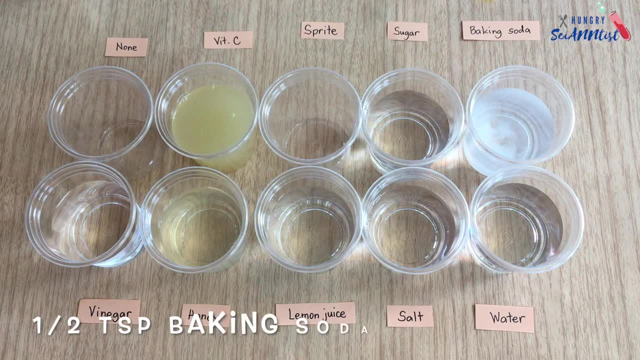 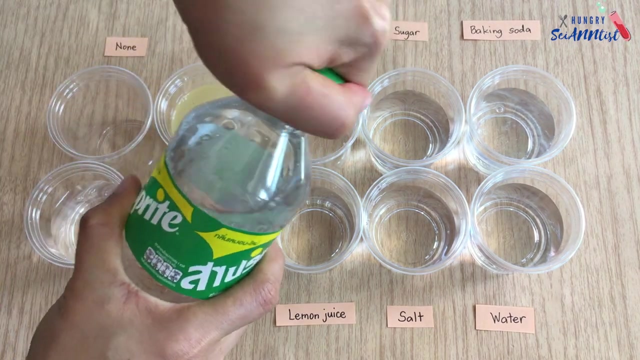 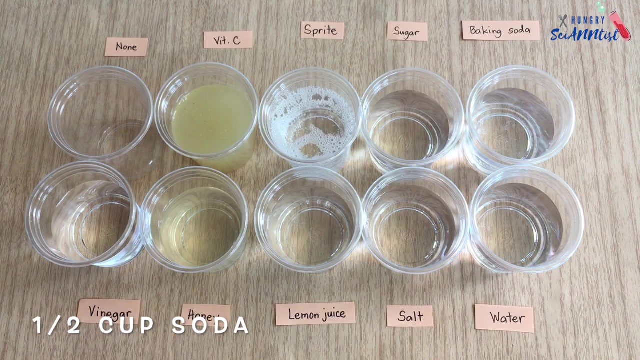 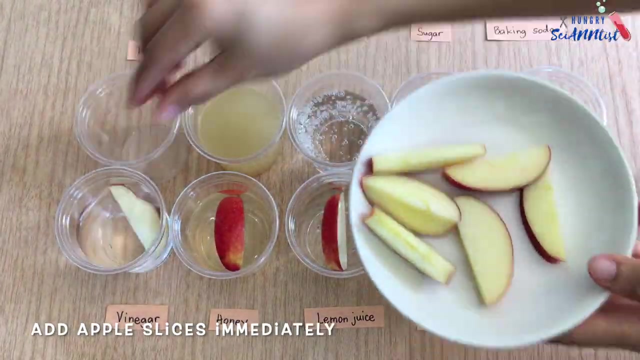 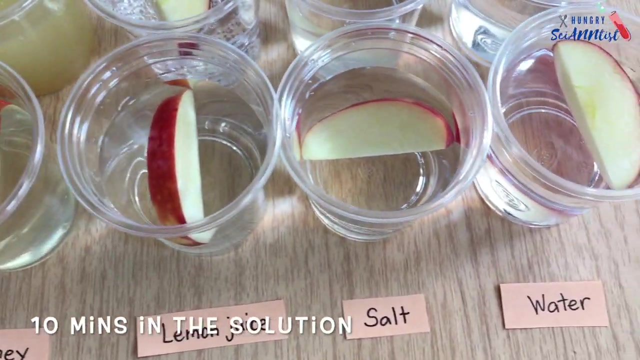 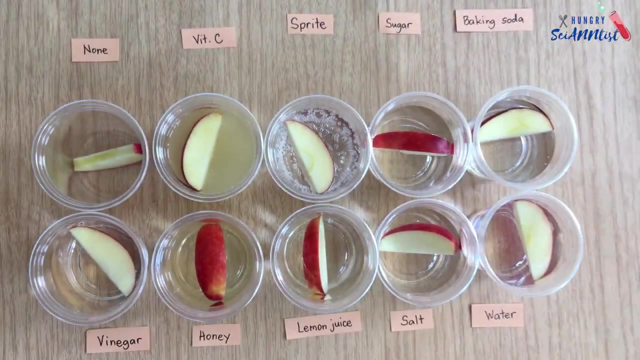 Half a teaspoon of baking soda, Soda or Sprite. The last cup will be no solution. Place some apples and put them immediately in the solution. Let them sit in the solution for 10 minutes. After 10 minutes, take them out of the solution. 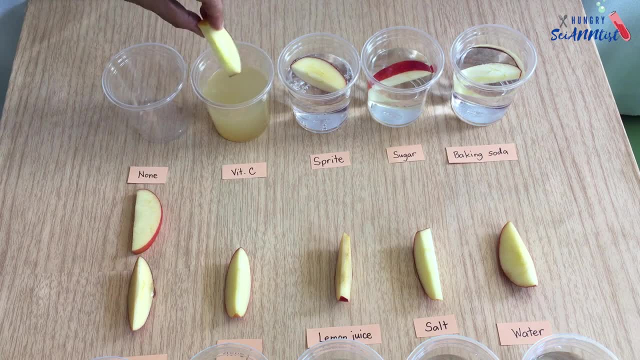 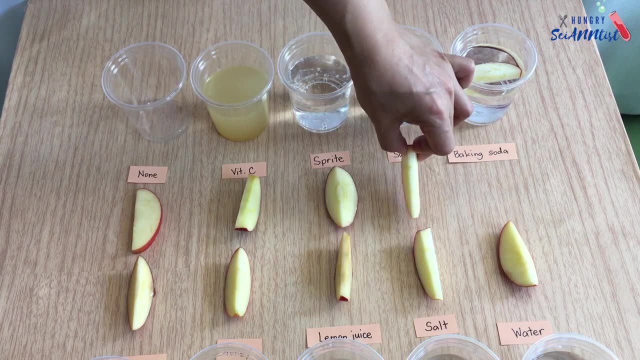 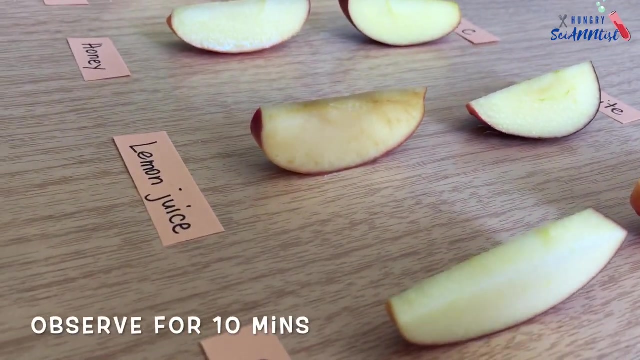 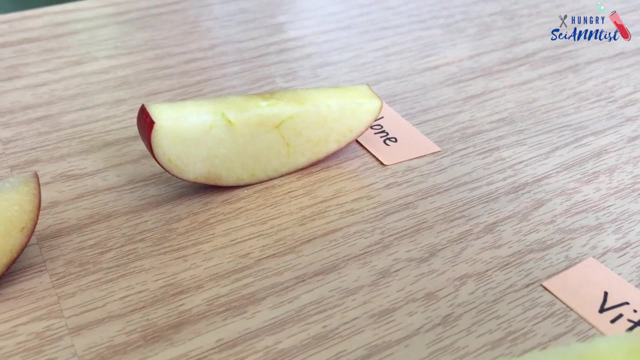 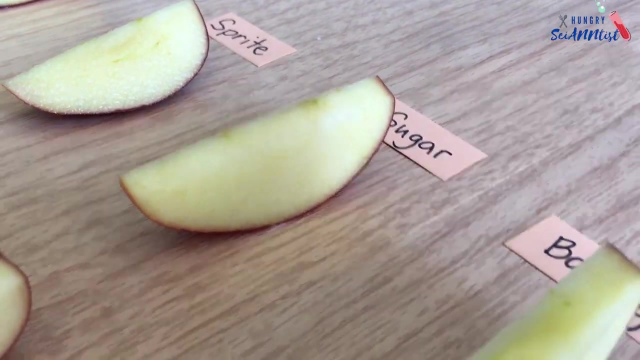 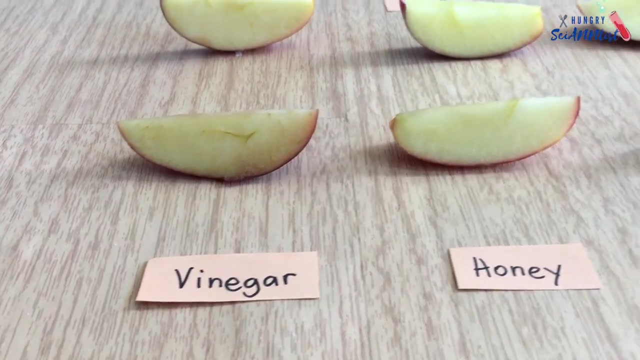 After 10 minutes, take them out of the solution. Observe for 10 minutes while exposed to air. Observe for 10 minutes while exposed to air. In my experiment, vinegar and lemon juice did not work well and salt solution shows. 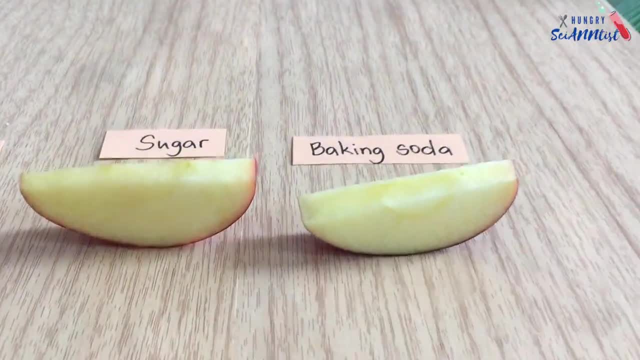 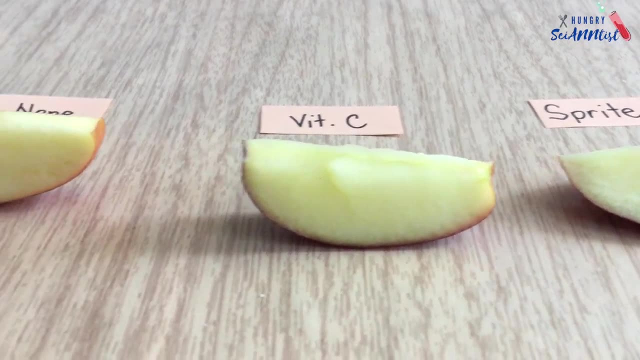 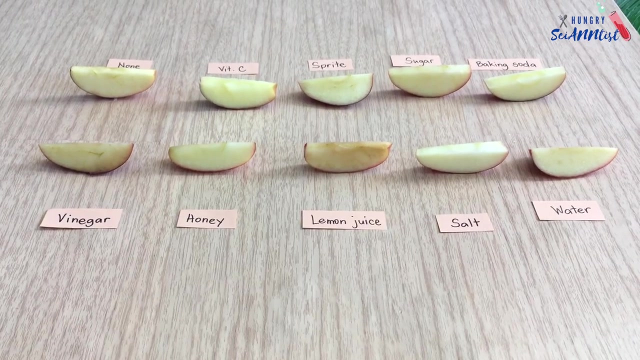 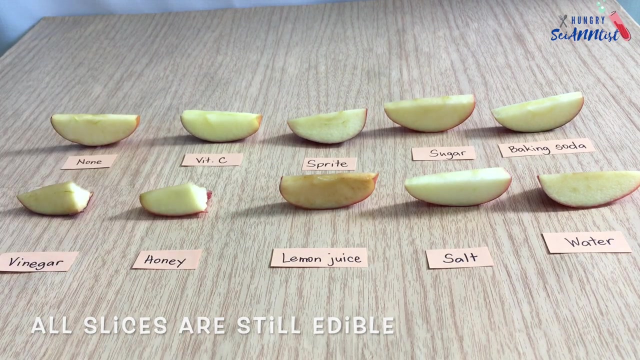 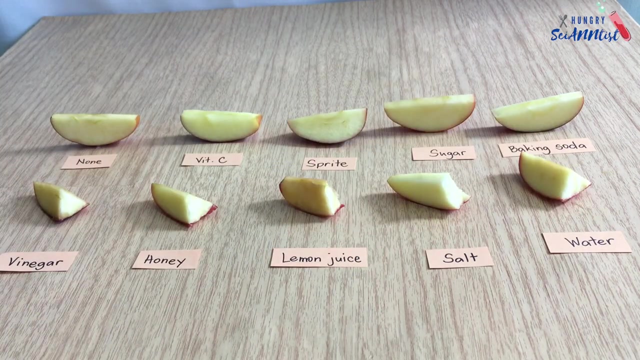 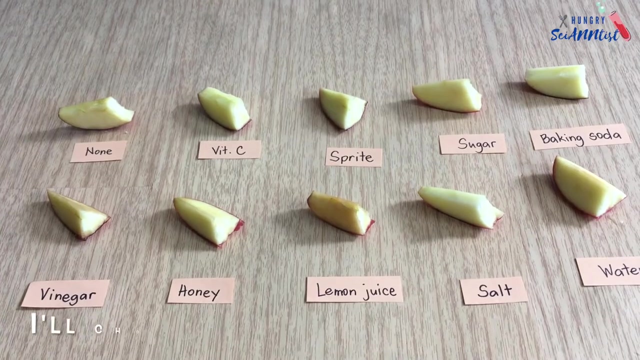 the best result. The apples turn brown in vinegar and lemon juice. Also, the taste is quite different. There are many other solutions able to keep the apples texture and crisp, but if I were to choose, I will choose salt solution. I found out that a salt water solution is the easiest and the best way to prevent apples. from browning. 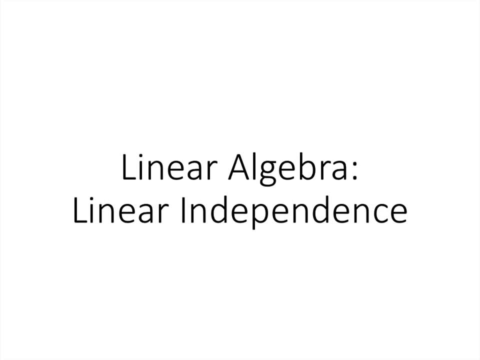 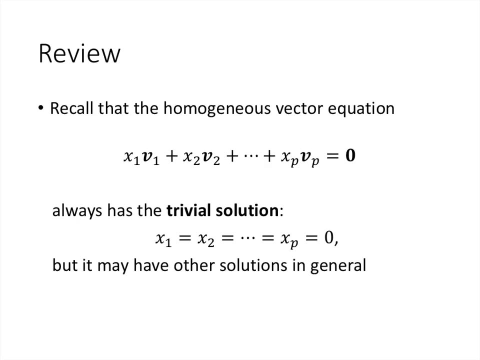 In this lecture we'll begin talking about a very important concept in linear algebra, and that's linear independence. So just to review, we've talked about what we called the homogeneous vector equation: x1v1 plus x2v2 and so on, through xpvp equals 0. So it's. 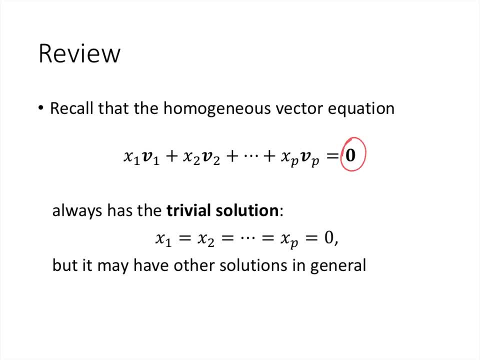 homogeneous because of the 0, and it's a vector equation because the vectors v1v2 through vp, those are all known, and the equation, the variables are x1, x2, up through xp, and we can write the solution to this equation as a vector. We're not going to do that in this lecture, but 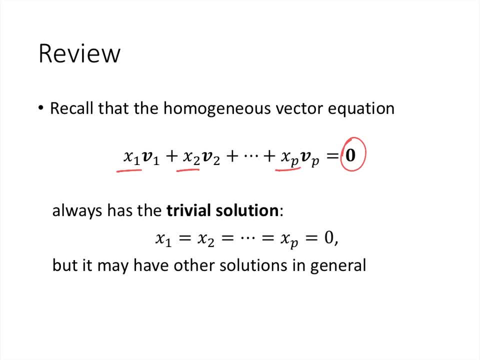 that's something to keep in mind going forward. But because it's a homogeneous equation, because we have this 0 on the right-hand side, one of the many solutions that this system could have is the trivial solution. If we put a 0 in for x1 and a 0 in for x2, all the way through a 0 in for xp.